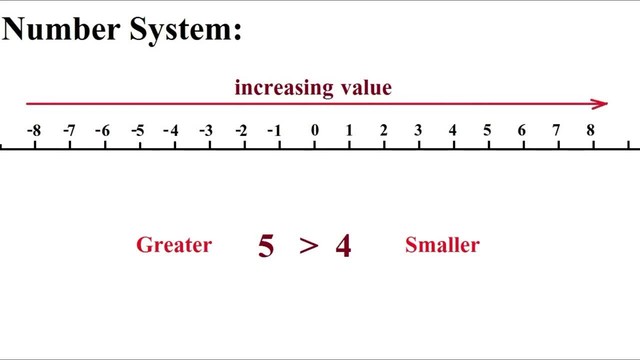 Thus 5 is greater than 4.. Now for the negative numbers: minus 5 and minus 4.. Minus 4 is greater than minus 5 because minus 4 comes right side of the minus 5.. How can we find the difference between any two numbers? 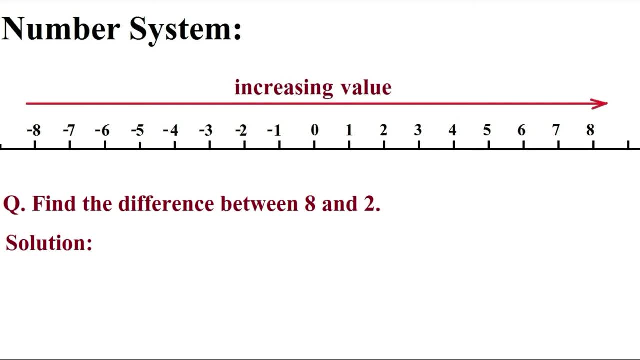 Suppose we need to find the difference between 8 and 2.. To find the difference between any two numbers, we must separate the smaller number from the bigger number. 8 is greater than 2.. So the difference will be 8 minus 2, and that is 6.. 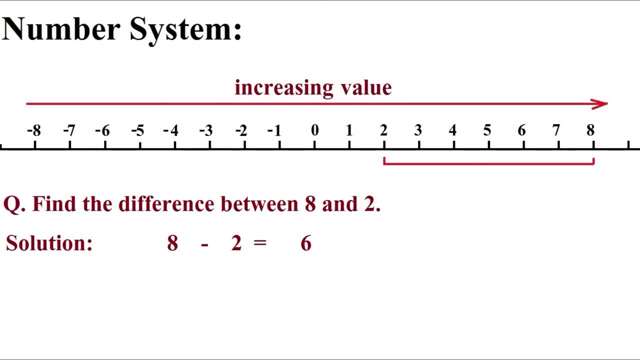 And you can see at the number scale, we have 6 units between 2 and 8. And if we need to find the difference between 8 and minus 1, simply 8 is bigger. Any positive number is always bigger than any negative number. 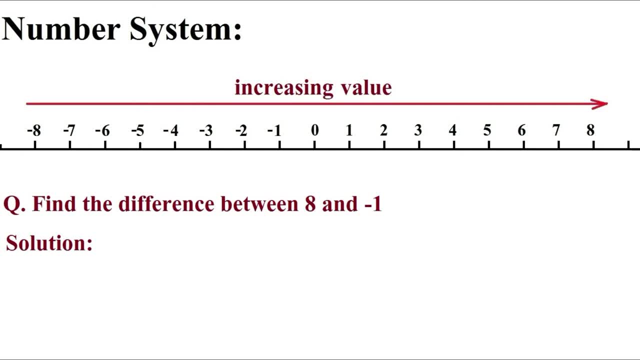 And also you can see, 8 comes right side to the minus 1 in number system. So greater minus, smaller it will be 8 minus minus 1.. Minus and minus become plus And 8 plus 1 equals to 9.. 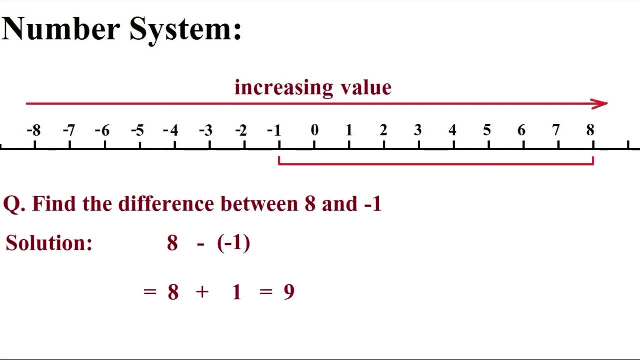 And at the number scale you can see we have 9 units, from minus 1 to 8.. Difference between 5 and minus 5, once again greater minus smaller. 5 minus minus 5, turns into 5 plus 5, equals to 10.. 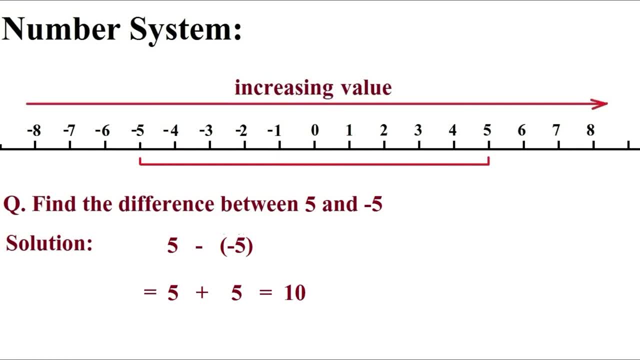 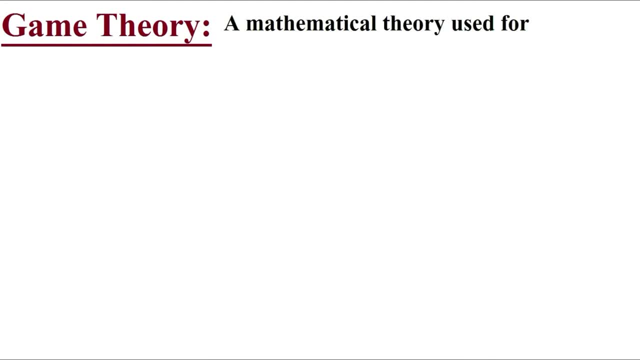 Here is the distance of 10 on number scale. So this is the difference between 5 and minus 5.. Now coming to the concept of game theory. Game theory is a mathematical theory used for competitive situations When competitors are trying to make decisions. 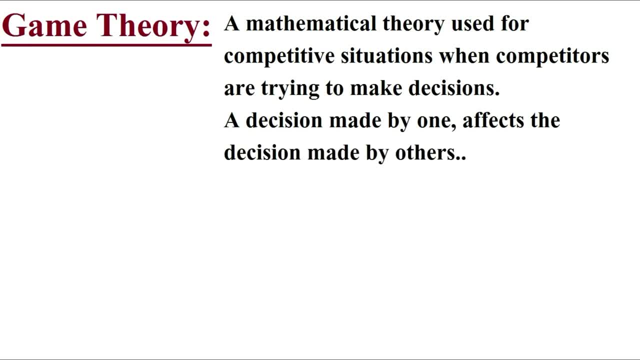 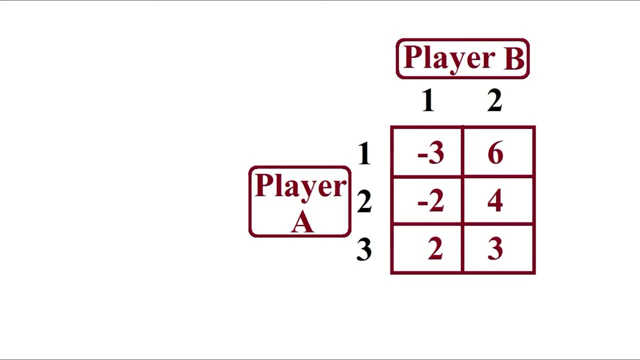 A decision made by any one competitor affects the decision made by others. This is the basic model of a game. A game occurs generally between two players, But sometimes number of players can be more than two. However, in this series we will learn only about two players' game. 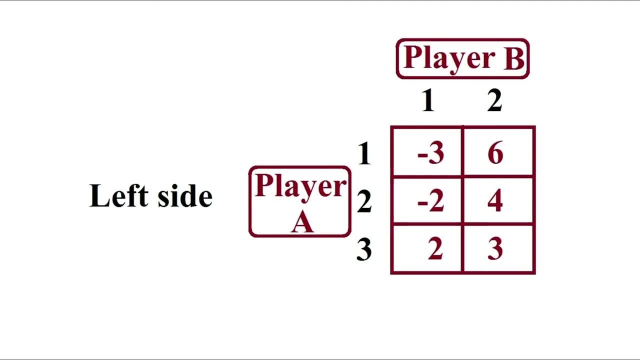 And their positions will always be left for one player and the top for other player. We cannot locate them at the bottom or the right side of the game, even if more than two players are involved. Each of the players will have some strategies: The action he can choose to play. 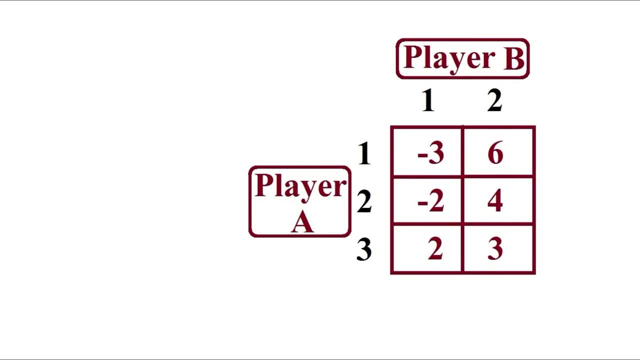 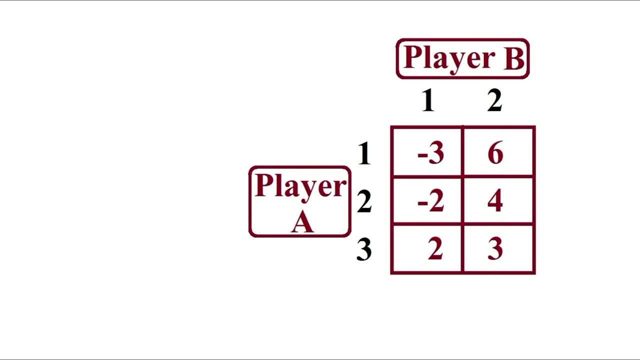 Similarly for the top-side player, all the columns can be considered as the available strategies In this game, the left-side player, player A, having three strategies, these three rows, While player B, top-side player, have only two strategies, both of the columns. 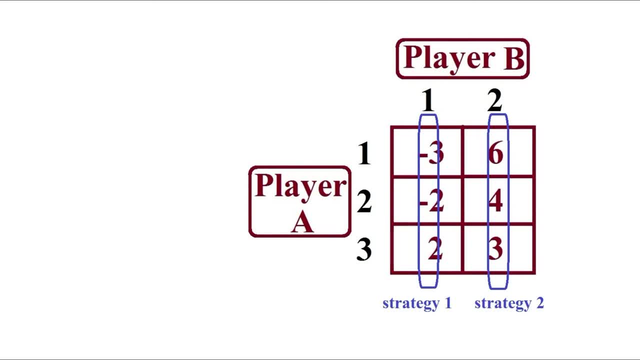 Number of strategies for both players means number of rows and number of columns need not necessarily be the same. Each square the game is made up of is called cell. Altogether they make the structure of any game. Now the very important concept: any positive value favors the left side player. 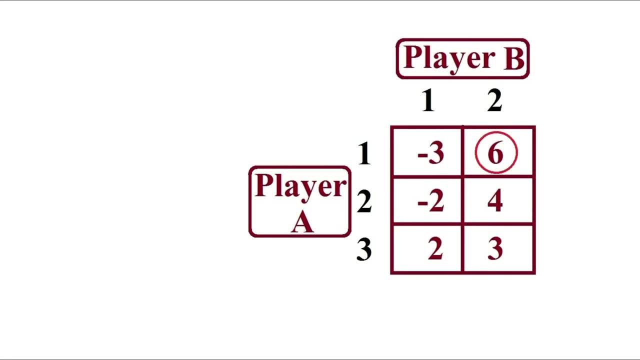 For example, this 6 or positive value indicating two factors: Gains or profit for player A by 6 points and, at the same time, loss for player B by the same value, 6 points- And any negative value favors the top side player. 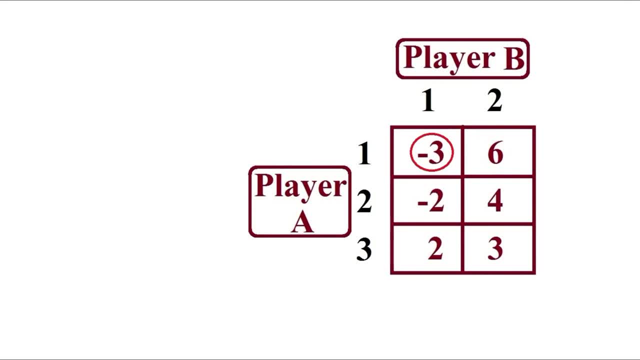 For example, this minus 3 or negative value, indicating two factors: Loss for player A by 3 points and, at the same time, profit for player B by the same value- 3 points. If player A gains profit, then at the same time player B incurs loss by the same amount. 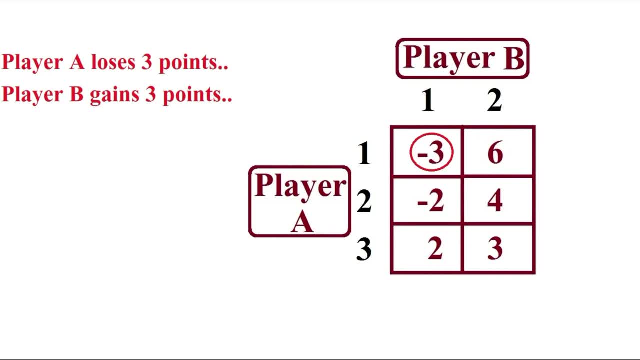 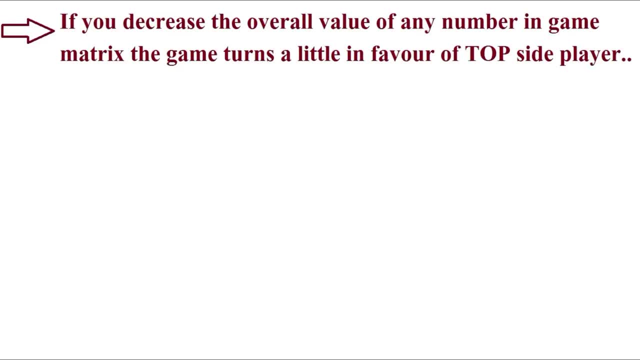 Similarly, if player B gains the profit, then at the same time player A incurs loss by the same amount. Now few other rules for a game. If you increase the overall value of any number in game matrix, the game turns a little in favor of top side player. 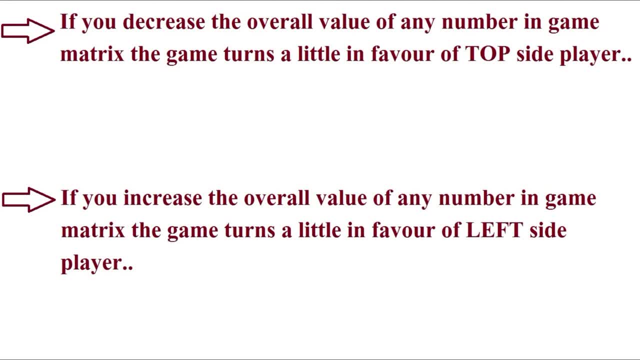 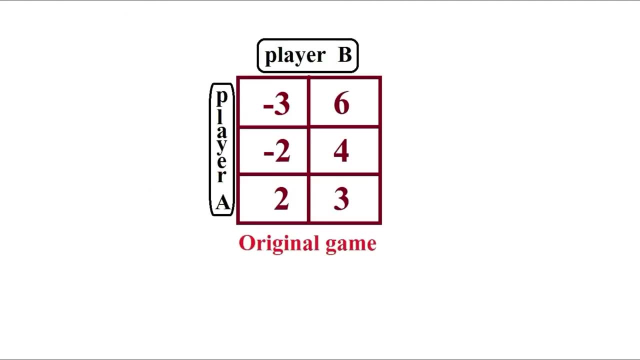 Similarly, if you increase the overall value of any number in the game matrix, the game turns a little in favor of left side player. Let's see how exactly. In this game we have a negative number minus 3.. We just prepared a new game. 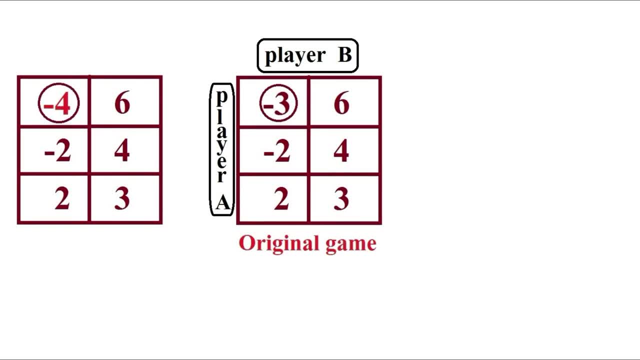 For comparison And placed minus 4 instead of minus 3.. And all the other values are same And you know very well minus 4 is less than minus 3.. Overall value means the value of any number with its positive or negative sign. 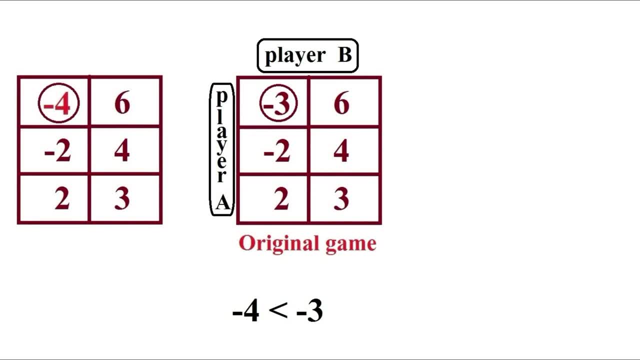 So we can say: value of one single number is decreased in this given game And that's why this game turns a little in favor of top side player, Player B. Similarly, if we increase the value In this game, we just placed minus 2 instead of minus 3.. 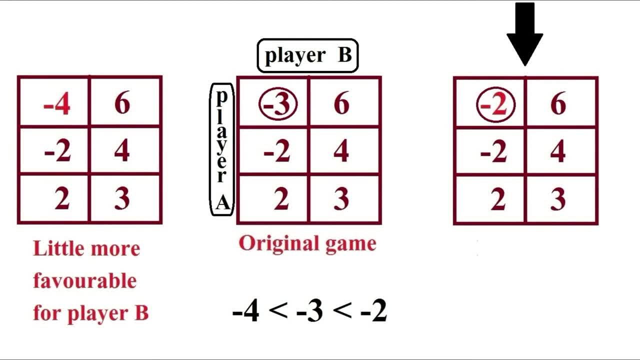 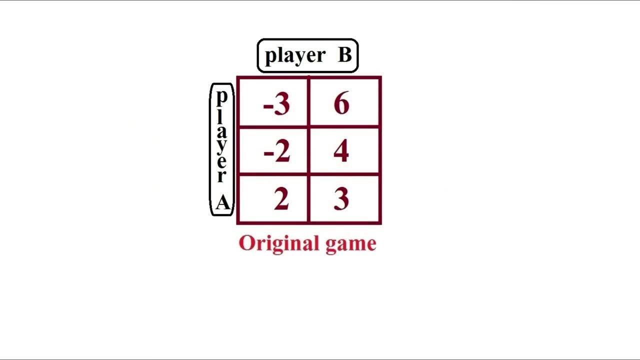 And minus 2 is greater than minus 3.. So by increasing the value, even for a single number, the game now turns in favor of player- A left side player- Compared to the original game. Change in any positive number will also results in the same manner. 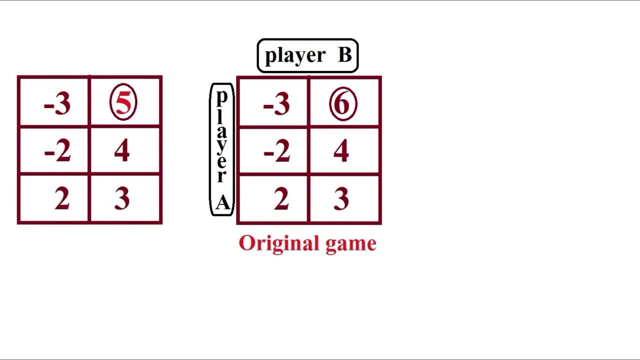 In this new game we just replaced a positive number, 6, by other number, 5.. So this means value of a single number is decreased. now 5 is less than 6. And that's why this game is little more favorable for player B than the original game. 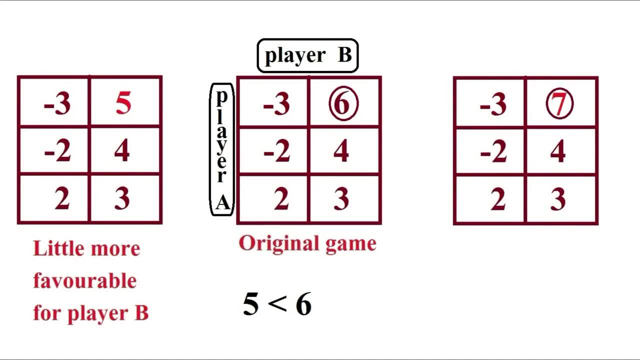 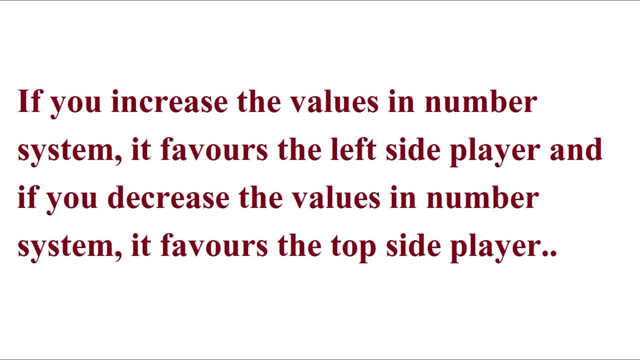 And if we replace the same number 6 with a bigger number 7.. Value increased now for a number And this game is little more favorable for player A than the original game. So not particularly for positive or negative values. But in general we can say if you increase the value in number system it favors the left side player. 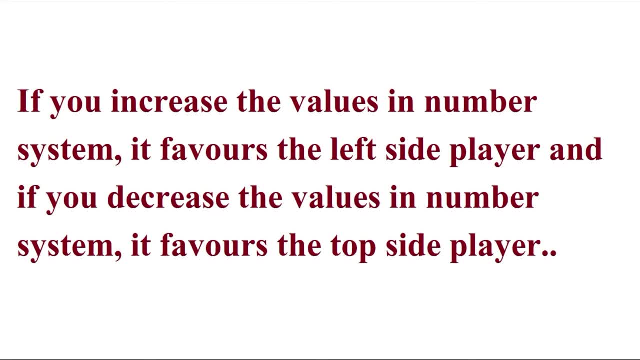 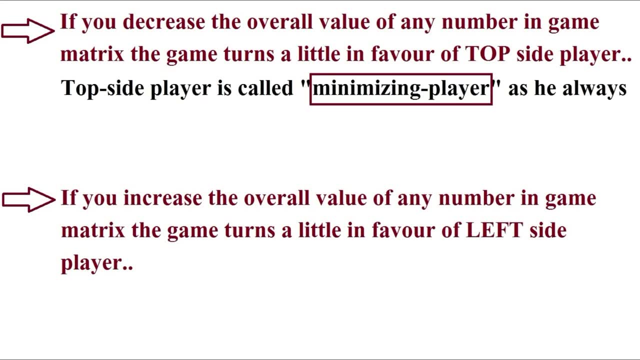 And if you decrease the values in number system, It favors the top side player. So we come to the conclusion that the top side player is a minimizing player And he will always try to minimize the values. And left side player is a maximizing player.